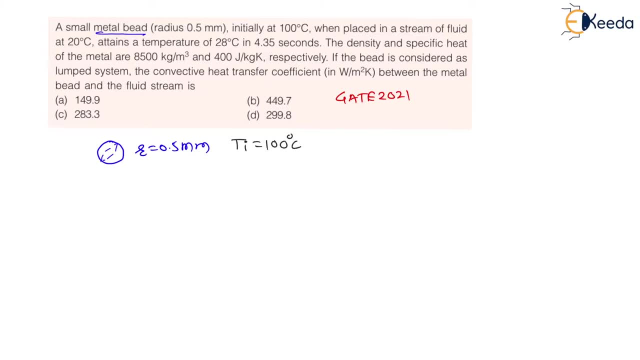 Therefore Ti is equal to 100 degree Celsius. Then, when placed in a stream of fluid at 20 degree Celsius, attains a temperature of 28 degree Celsius in 4.35 seconds. Now the fluid stream temperature is nothing, but we are representing with T, infinity, which is given 20 degree Celsius. 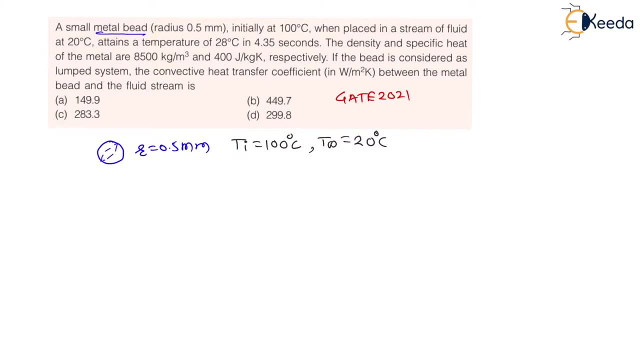 And this metal bead. when you are kept in this stream- temperature fluid temperature of 20 degree Celsius, then its temperature becomes 28 degree Celsius in time- 4.35 seconds. Therefore, temperature becomes 28 degree Celsius in time T- 4.35 seconds. 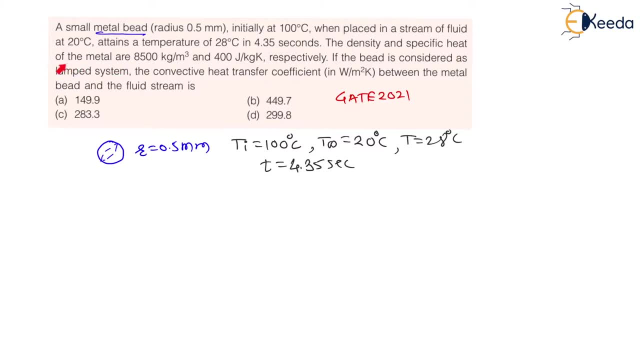 Then the density and specific heat of the metal bead are Now: density is given, specific heat Cp is given. Therefore, rho is given 8500 kg per meter cube and specific heat Cp is given, 400 joule per kg kelvin. Then, respectively, if the bead is considered as lumped system, 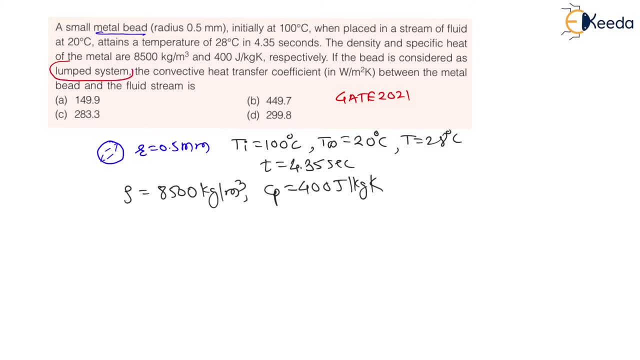 Now this is very important. Here they are considering as a lumped heat capacity system Means we can use the formulas of lumped system. Then the convective heat transfer coefficient in Watt per meter square kelvin between the metal bead and the fluid stream is: 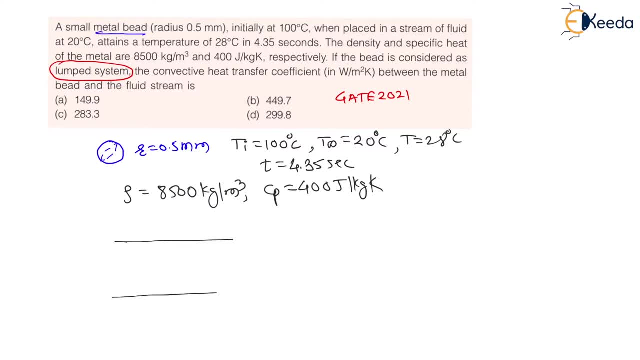 Now what is happening here? Let us say there is a stream like this. This is the stream flowing Now. the temperature of stream is T, infinity, and convective heat transfer coefficient of this fluid stream is Eh. Now, in the direction of this flow, a metal bead is kept. 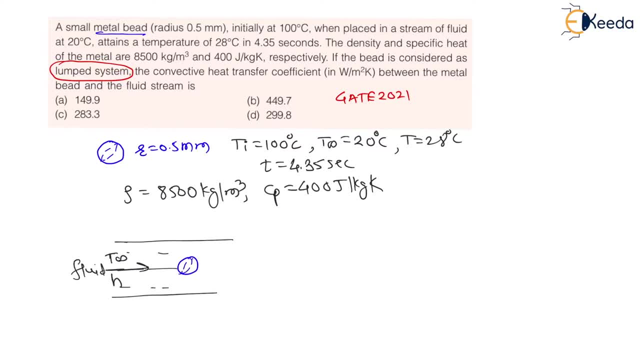 Having some radius R And my dear students, the initial temperature of this bead is Ti. Now, after time T, what will be the temperature? T? After time T, the temperature will be T. Then what is this convective heat transfer coefficient, Eh, if density and Cp are given. 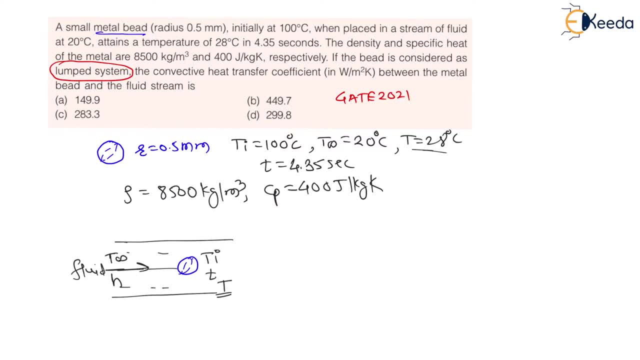 Now for such cases, assuming lumped system, As they have mentioned, consider lumped system. For lumped system we have derived formula that is temperature T minus surrounding fluid. temperature T infinity divided by Ti minus T infinity Is equal to e, to the power minus Ha divided by rho V Cp into time T. 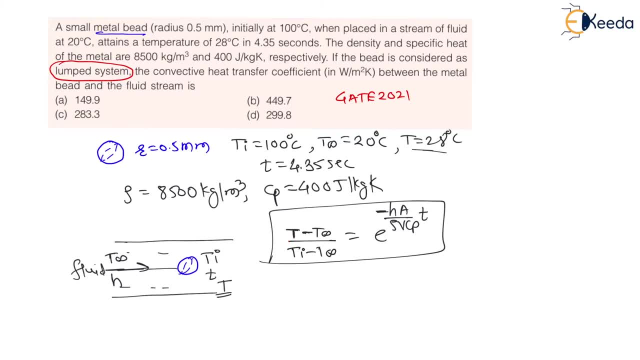 This formula we have derived, Where T is the temperature, after some time, T, T infinity is the fluid temperature. Ti is the initial temperature of this metal bead. Eh is the convective heat transfer coefficient between this metal bead and surrounding fluid. A is the surface area of this bead. 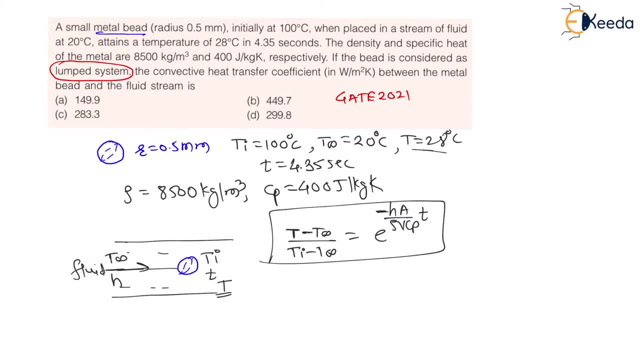 Rho is the density of this bead, V is the volume of this bead, Cp is specific heat of this bead And T is the time in second. Now the same formula if I consider logarithmic function or alien function, on both sides. 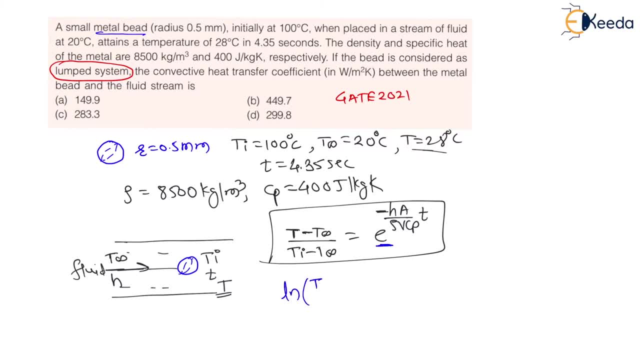 To remove this exponential function, Then it will become alien of T minus T infinity. divided by Ti minus T infinity Is equal to minus Ha divided by rho V, Cp into T. Now, my dear students, let us find this area divided by volume for this sphere. 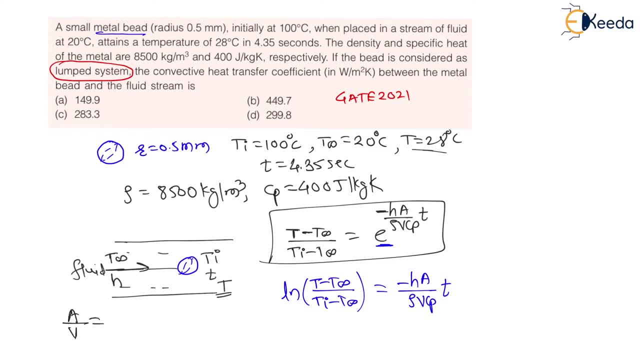 If I find here area divided by volume for this sphere, Area of sphere is 4pi R square And volume is 4 by 3. 4 by 3 pi R cube. Therefore, here in this 4pi will get cancelled. 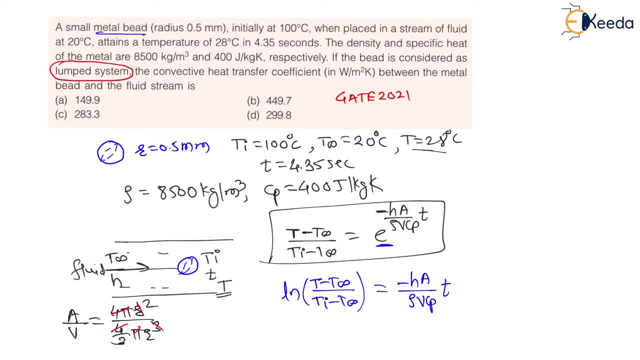 R square. R square will get cancelled. Then this area divided by volume, Area divided by volume of sphere, will become 3 divided by R, Right? So, my dear students, here, this area divided by volume, we will replace with 3 by R. 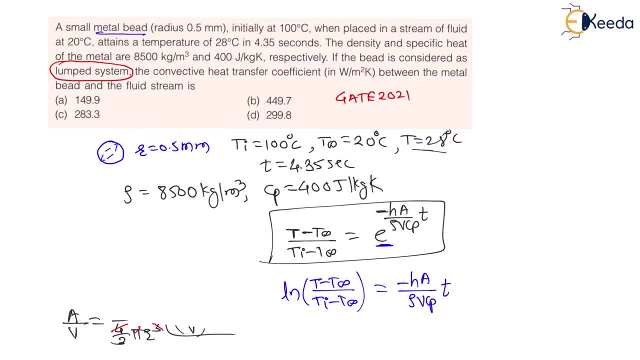 So let us replace this: Instead of this area divided by volume, we are going to put here 3 divided by R. Therefore, the formula will become alien of T minus T. infinity divided by Ti minus T infinity Is equal to minus H into T divided by rho Cp. 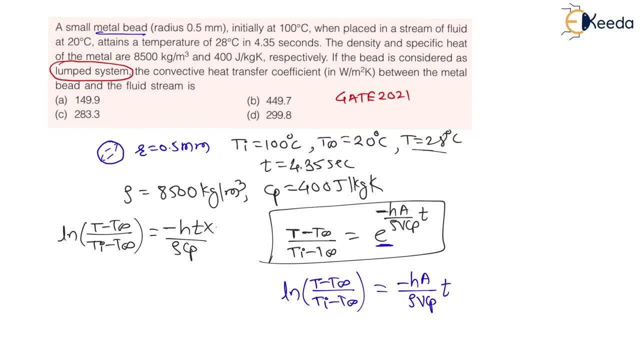 And this area divided by volume is 3 by R. Therefore, into 3 divided by R, Right, So let us put the values. Therefore we will get alien of T is nothing but T is given 28 degree Celsius, Therefore 28.. 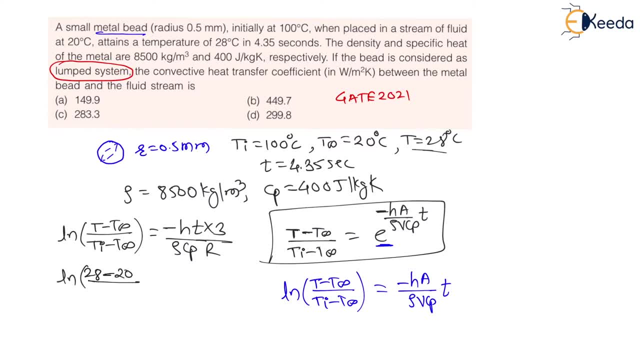 Minus T infinity is 20.. Divided by Ti is 100.. Minus T infinity is 20.. Is equal to minus H. into time is Here 4.35 seconds. Therefore, 4.35 seconds into 3..